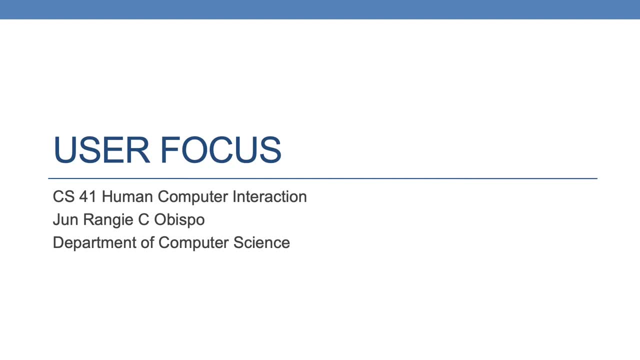 Now we'll talk about user focus. As we've already said, the start of any interaction design exercise must be the intended user or users. This is often stated, as know your users. Note that much of traditional user interface design has focus on a single user. 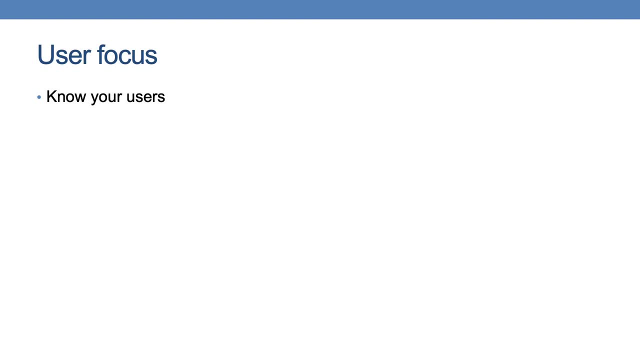 It is important to be aware that there is rarely one user of a system. Almost every system has an impact beyond the person immediately using it. Think about a stock control system. The warehouse manager queries the system to find out how many 6-inch nails are in stock. just a single user. Why did he do this? Perhaps a salesperson? 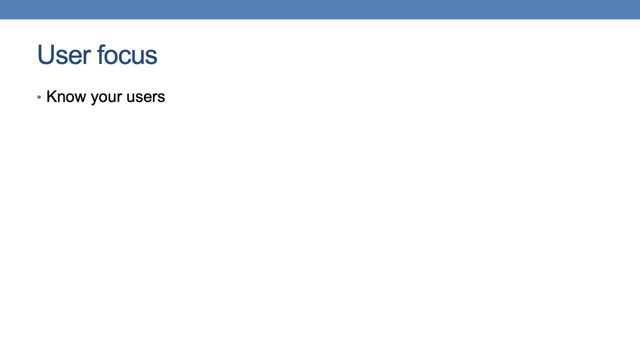 has been asked to deliver 100,000 6-inch nails within a fortnight and wants to know if the company is able to fulfill the order in time. So the act of looking at the system cannot be applied to a single user. A different system might help to provide a 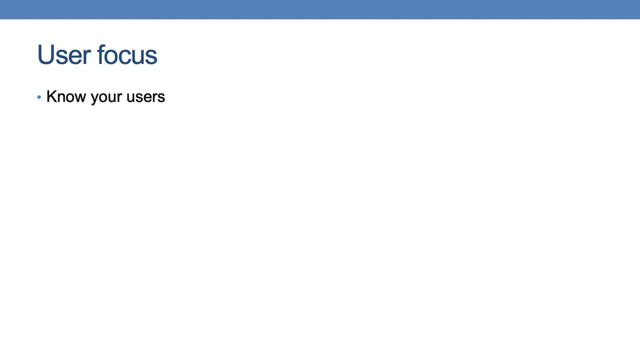 stock control system involves the warehouse manager, the salesperson and the client. Over time, many people are affected directly or indirectly by a system, and these people are called stakeholders. Obviously, tracing the tenuous links between people could go on forever and you need to draw boundaries as to whom you should consider. This depends. 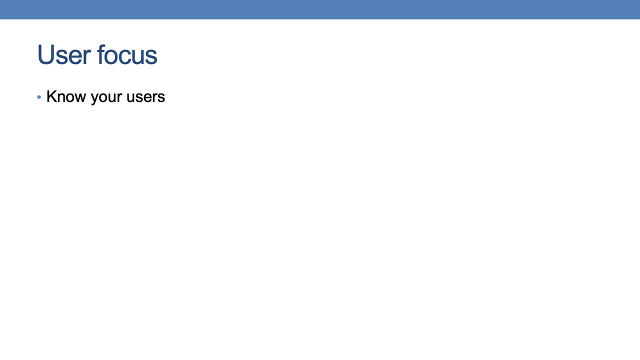 very much on the nature of the systems being designed, but largely requires plain common sense. So how do you get to know your users? First thing, find out who your users are, their demographic, Are they old, young, experienced, novice, etc. It may not be obvious who the 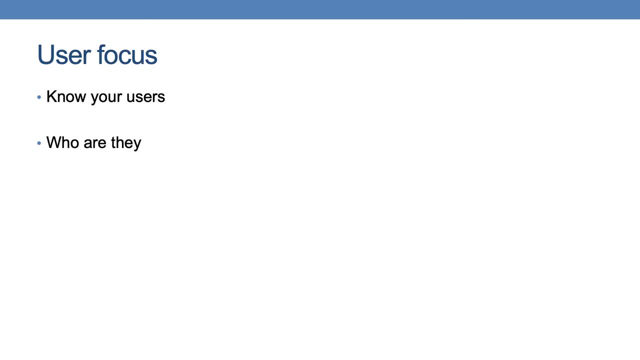 users are, but you'll get to find out more as you know more about the system and its context. This question becomes harder to answer if you are designing generic software such as word processor, as there are many different users with different purposes and characteristics. 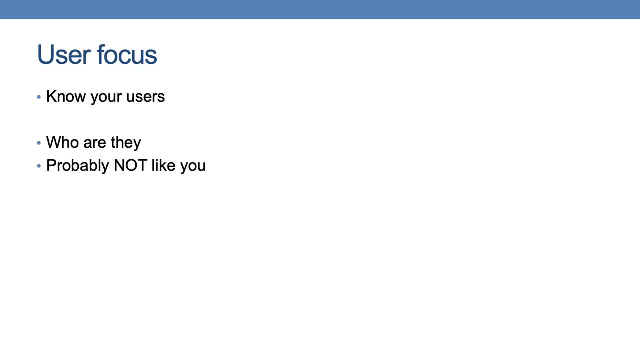 Second, assume that your users are probably not like you. When designing a system, it is easy to design as if you were the main user. You assume your own interests and abilities. It may be obvious for you, but not for others. Last but not least, be considerate of the tasks. 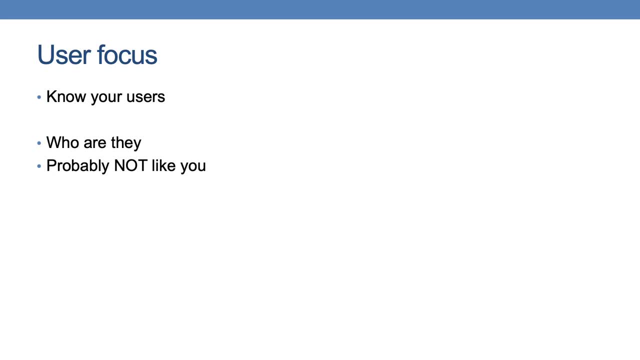 To follow-up with that assumption, the best thing to know your users is to ask them. This can take many forms—structured interviews, open-ended discussions or bringing the potential users fully into the design process—called participatory design, By involving users throughout. 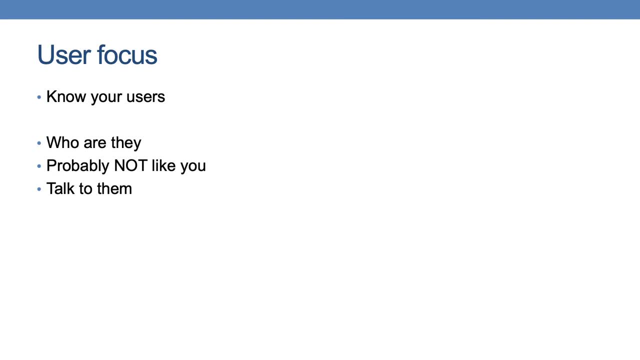 a design process, it is possible to get a deep knowledge of their work contexts and needs being involved. a secondary motivational effect arises. Users come to own the design and become champions for it once deployed. Recall that a system must not only be useful and usable. 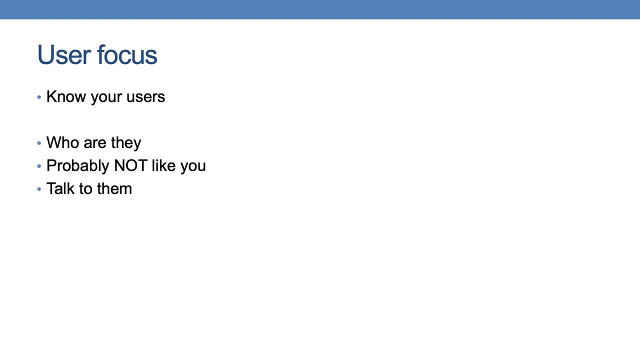 but also used. Although what people tell you is of utmost importance, it is not the whole story. A professional in any field is very practiced and can do things in that domain. An academic in the same field may not be able to do things, but she knows about the things in that. 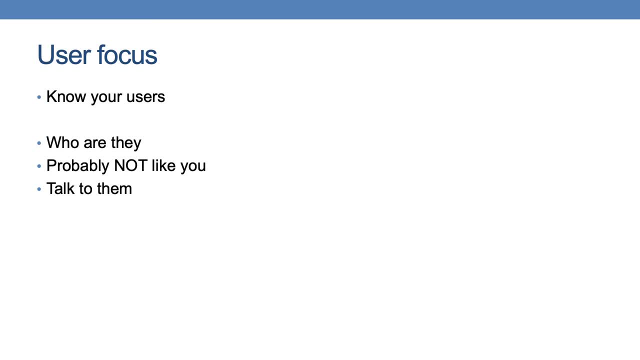 domain. These are different kinds of knowledge and skill. Sometimes people know both, but not necessarily so. The best sports trainer may not be the best athletes. the best painters may not be the best architects, and because of this it is important to watch what people do as well as hear. 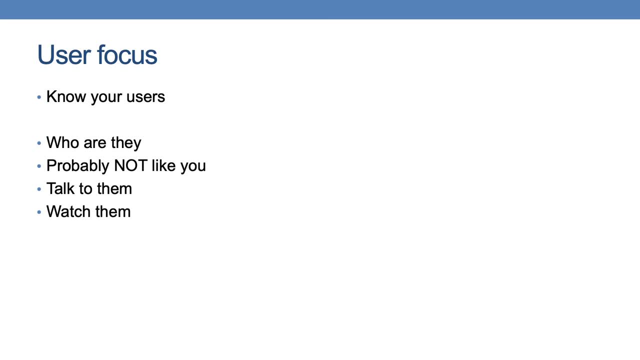 what they say. Even if you would like to learn more about the world of art, you may not be able to do it without the help of a professional. If you would like to involve many users throughout your design exercise, this will not always be possible. It may be too costly, It may be hard to get time with. 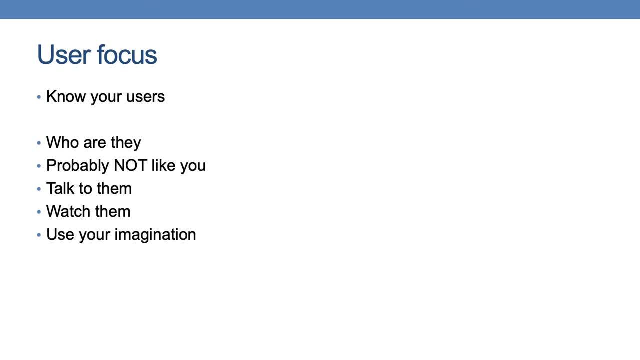 them. It may be that there are just too many. However, even if you cannot involve actual users, you can at least try to imagine their experience. Now, this is very dangerous. This issue is not what you would do in the user's shoes, but what they would do. This requires almost a couple of steps. First, you need to know what you are doing. Second, you need to know what you are doing. Third, you need to know what you are doing. And finally, you need to know the design. The design is a combination of an individual and an individual's approach to the design. 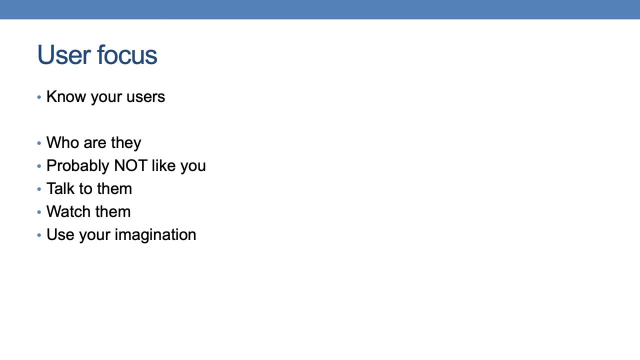 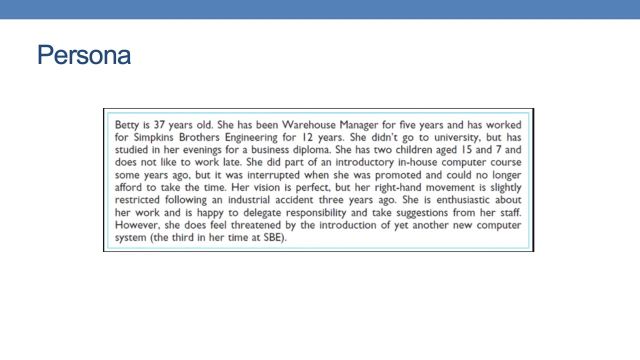 The design is a combination of an individual's approach to the design. One method that has been quite successful in helping design teams produce user-focused design is a persona. A persona is a rich picture of an imaginary person who represents your core user group. Consider the figure text shown. The figure text gives an example. persona of Betty. 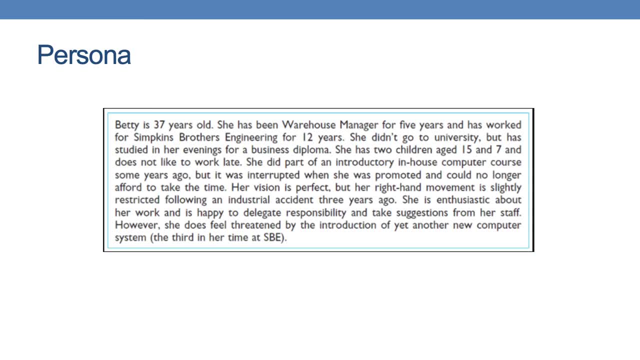 the warehouse manager. A design team will have several of the following methods: personae covering different types of intended users and different roles. The personae will themselves be based on studies of actual users, observation, etc. When a design solution is proposed, the team can ask: how would Betty react to this? 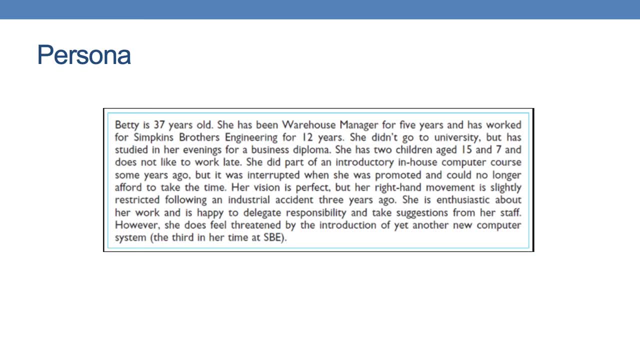 The detail is deliberately more than is strictly necessary, but this is essential. It is only by feeling that Betty is a real person that the team can start to imagine how she will behave. 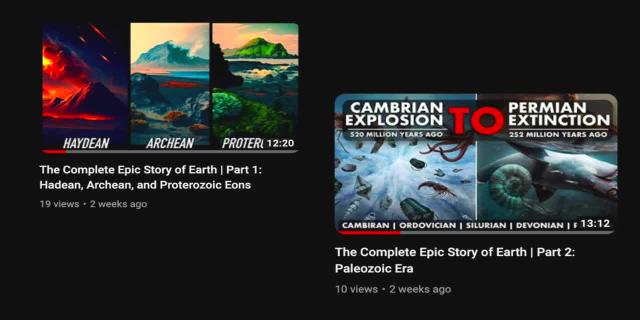 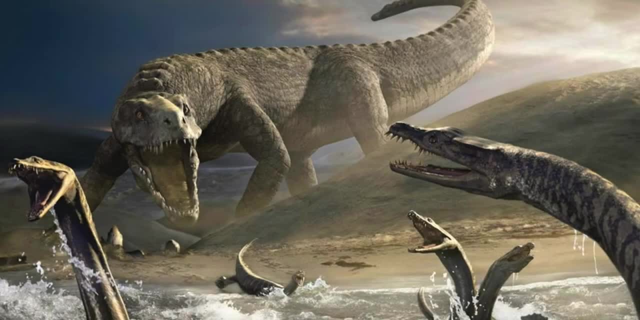 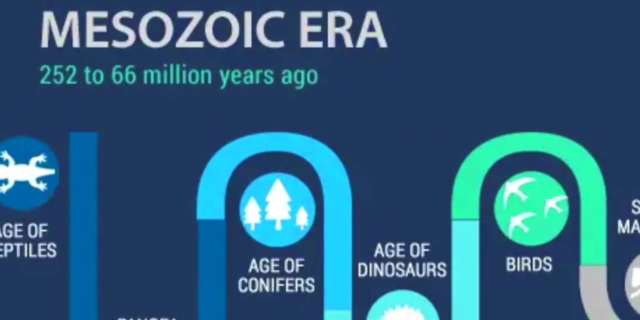 In the previous videos of our series, we explored the fascinating events that shaped the Earth's history leading up to the Mesozoic era. Now we embark on a journey through the Mesozoic era, often referred to as the Age of Dinosaurs, This era lasting from approximately 252 million years. 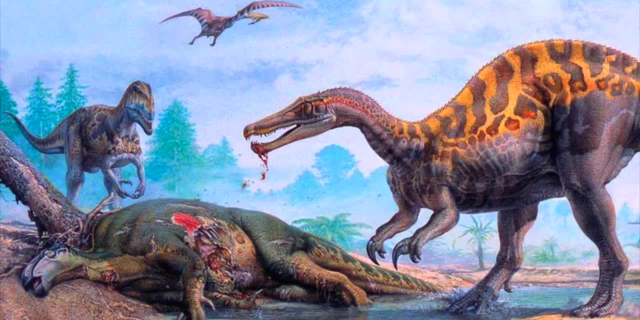 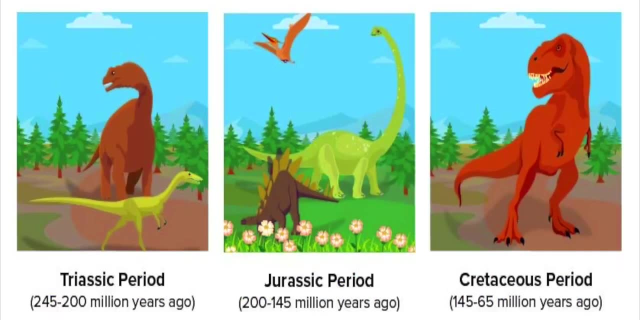 ago to 66 million years ago witnessed remarkable changes in the planet's life forms and environments. Triassic period- The Mesozoic era, is divided into three main periods, and in this video we will delve into all three of these periods, the first one being the Triassic period. 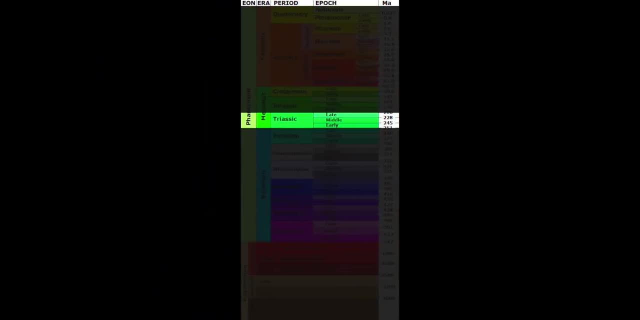 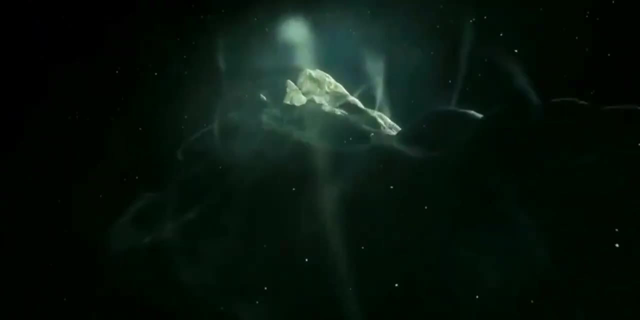 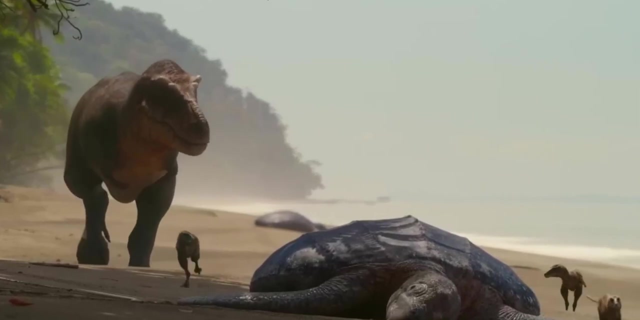 Lasting from approximately 252 million years ago to 201 million years ago. the Triassic period marked a significant transitional phase. following the mass extinction event at the end of the Paleozoic era, Life on Earth began to recover and evolve once again, paving the way for the 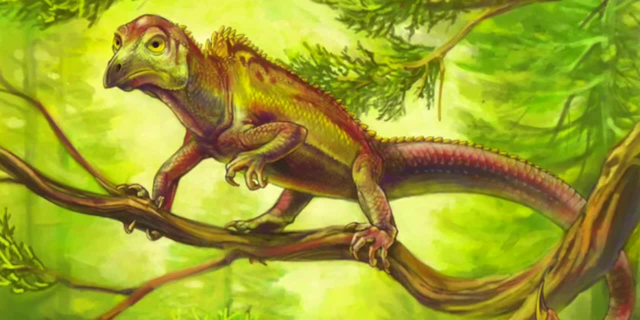 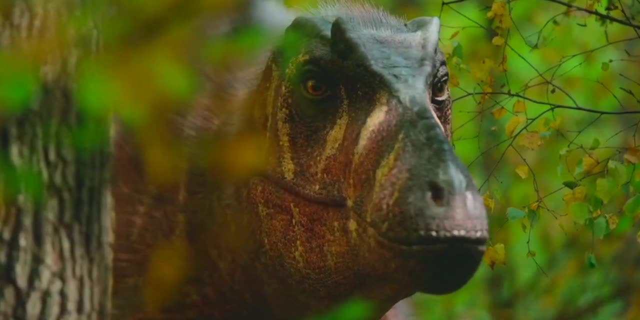 rise of the Mesozoic era. The Mesozoic era was a period of great change for the planet, of new and diverse species. During the Triassic period, reptiles took center stage, diversifying into a wide range of forms. These reptilian pioneers inhabited diverse habitats. 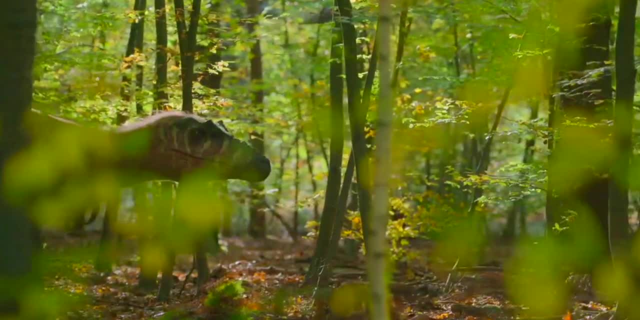 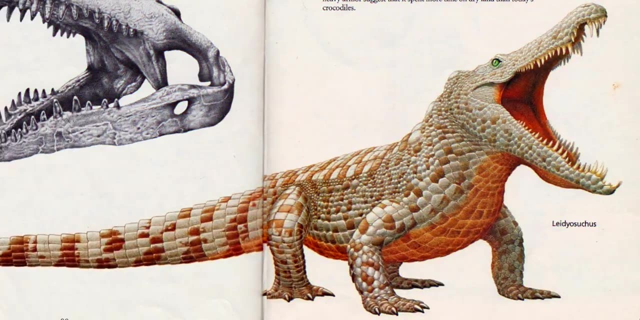 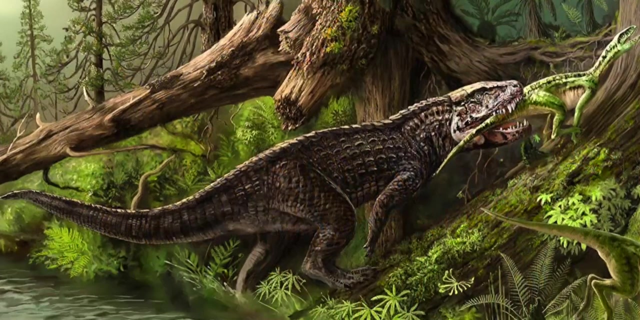 from the land to the sea and even the skies. The Triassic period witnessed the emergence of the first dinosaurs, representing a crucial milestone in Earth's evolutionary history. One notable group of reptiles that thrived during this period were the Archosaurs, which included formidable predators like the Phytosaurs and Rawisuchians.